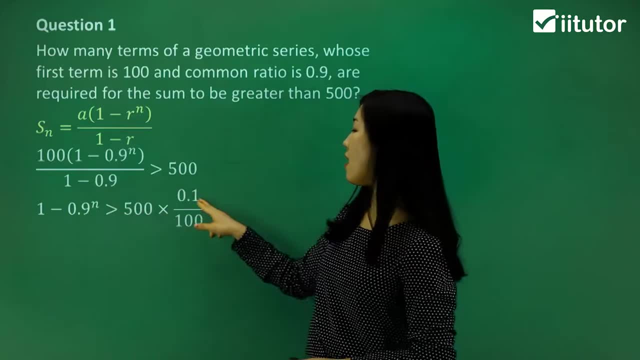 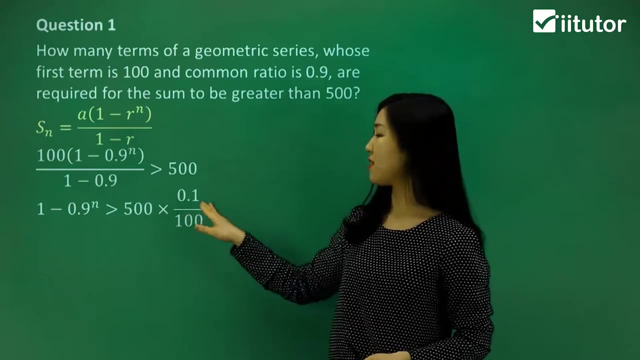 Alright, guys. so multiply by the denominator 0.1, and then divide by the coefficient of 100.. And then I'm going to make my left-hand side a little bit more simple, isn't it? And if you can simplify this right-hand side, for me, guys, you should probably get 0.5.. 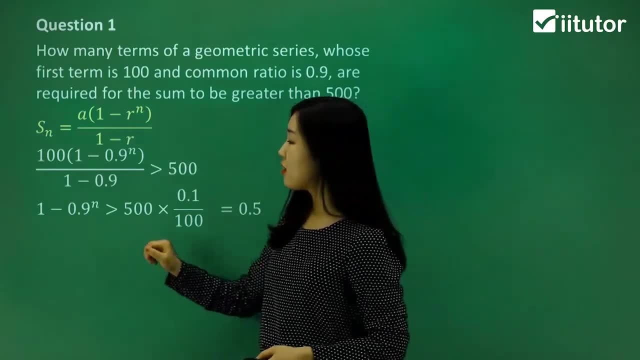 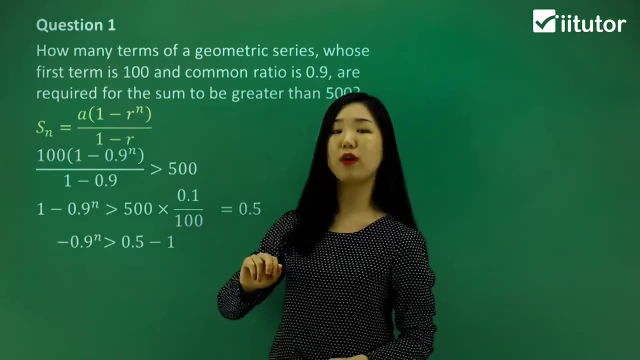 So just simplify on your way as you go. Now the 1,, I'm going to subtract it over to the other side, so it's 0.5 minus 1.. And on the left-hand side I'll have my negative 0.9 to the power of n left. 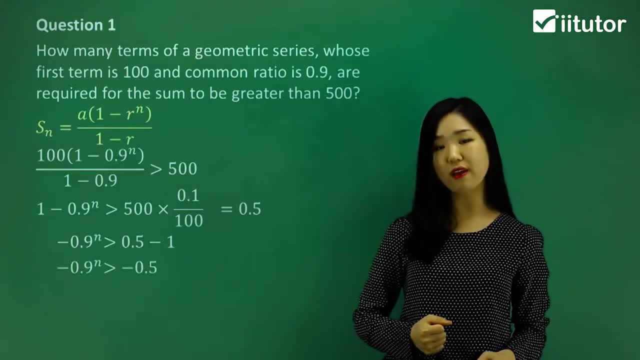 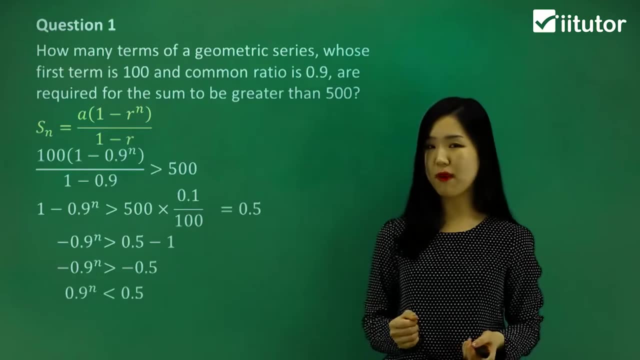 0.5 minus 1 is negative 0.5.. Now, guys, to get rid of the negatives on both sides, I have to make sure I switch the sign. Yeah, when we divide or multiply by a negative, which I'm doing now, we flip the sign around. 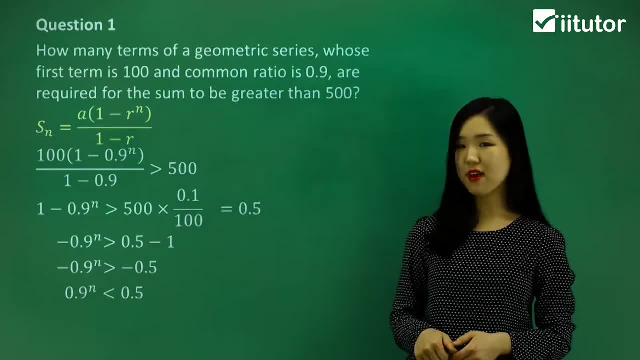 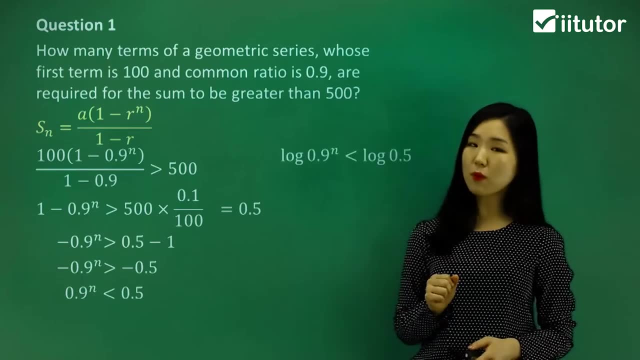 So 0.9 to the power of n is less than 0.5.. So we have to solve for n guys, but n is on the power. So the most ideal way is to use logs. So I'm going to log both sides just like this. so put the log function on both sides. 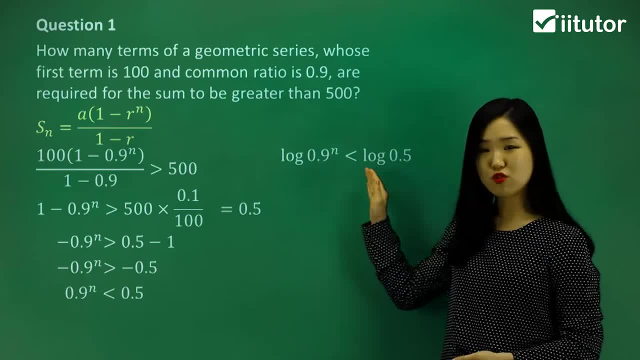 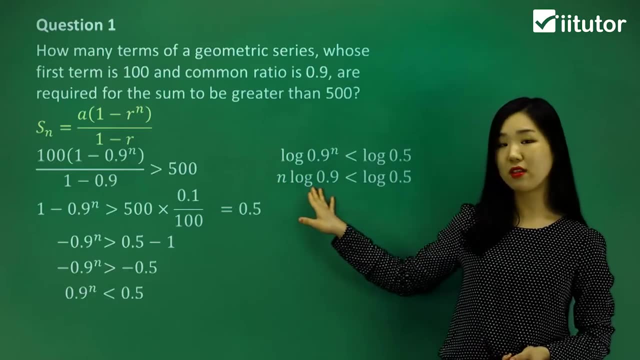 And now that I've done that, the power n, we can drop it down to the front like this, can't we? So the n, just drag it down to the front Now. what I'll do next is divide by the log 0.9 onto the other side, and then I'll have n by itself left. 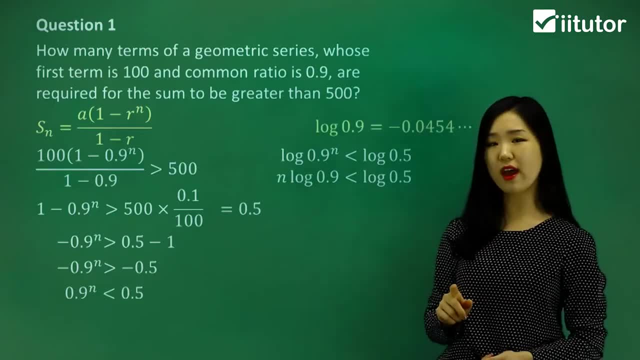 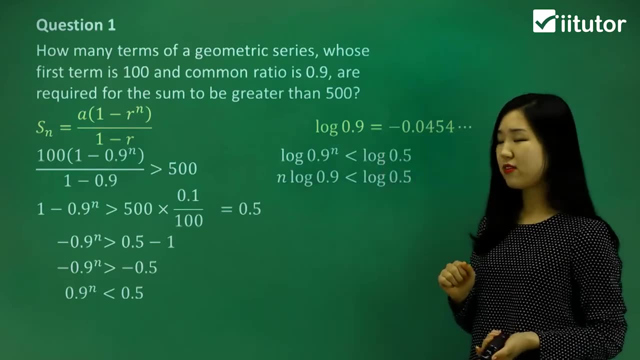 But guys, just remember this for me: For log 0.9, if you put it in the calculator you'd get a value of something like negative 0.04.. It's going to be a negative number. So usually with the numbers that are less than 1, we usually get log functions as a negative outcome. 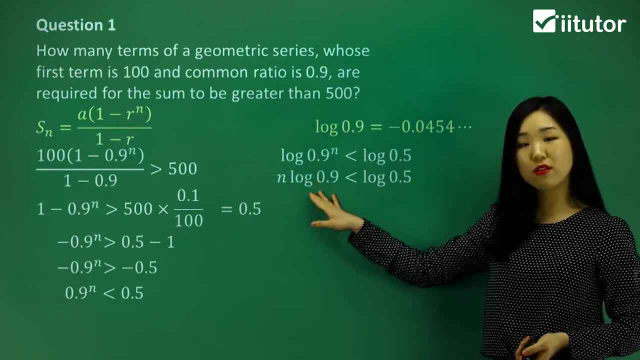 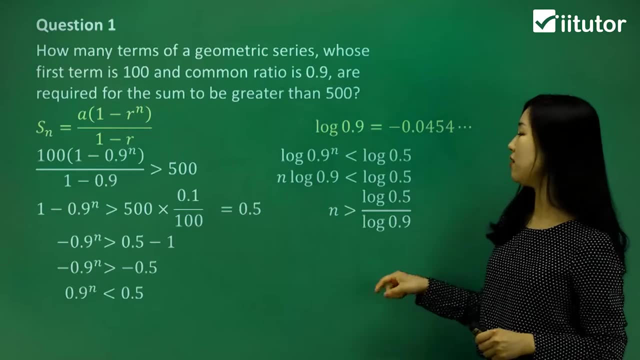 So try to keep that in mind. So if this is a negative number and I want to divide by a negative number, we have to switch the sign. So remember, when we divide by a negative, we switch the sign around. So we know that this is a negative number, so I change the inequality sign around, like that. 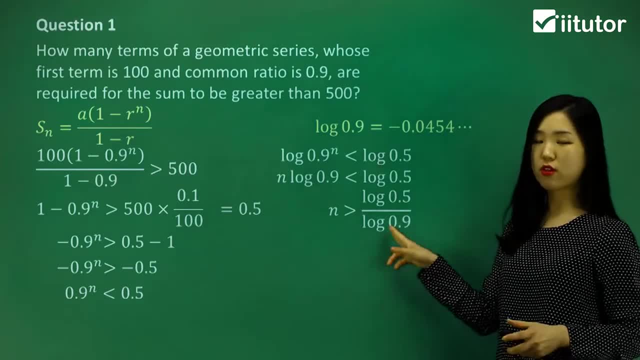 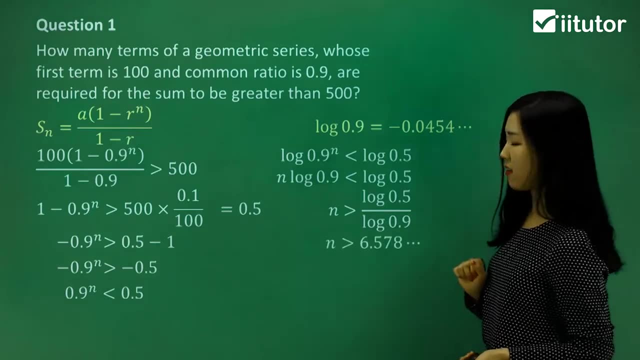 So negative. Now, log 0.5 divided by log 0.9, put it into the calculator for me and you'll get a value of 6.578, something like that. And then we want n. n must be a whole number, isn't it guys? 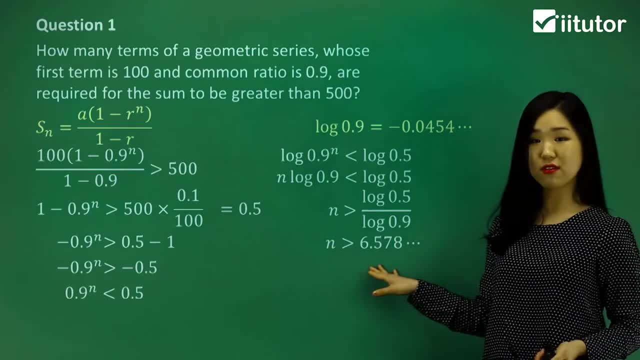 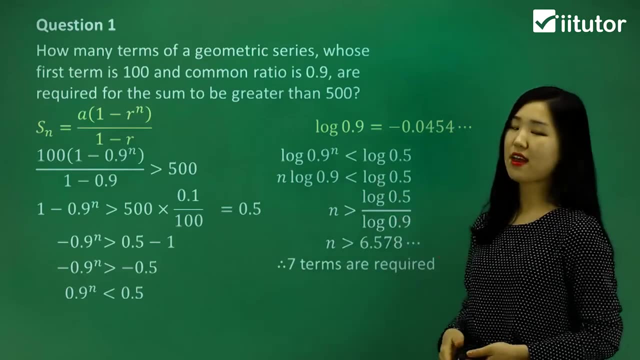 So what's the first whole number greater than 6.578, guys, It must be 7.. So we can say that the 7 terms are required to make the sum greater than 500..